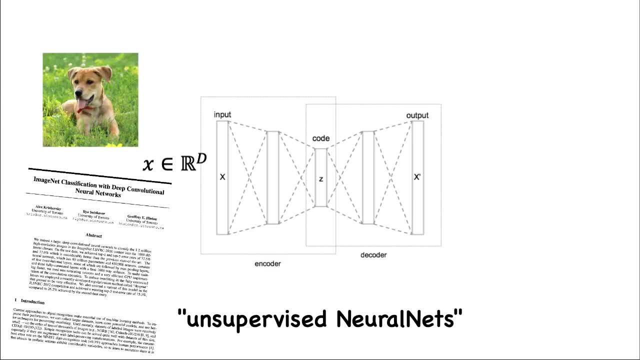 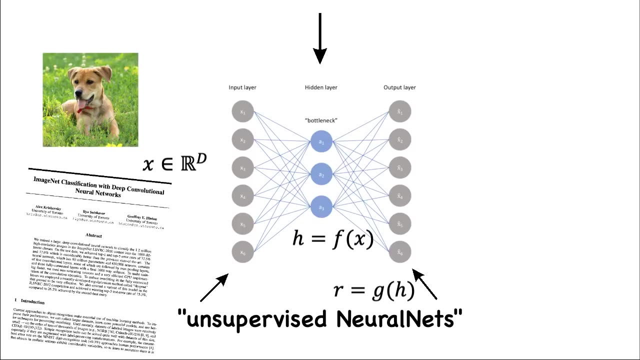 networks. Usually you wouldn't associate neural nets with being unsupervised, but today you will. The architecture consists of three parts: an encoder, a bottleneck and a decoder. At the simplest level, we can have a layer of fully connected neurons for each part. 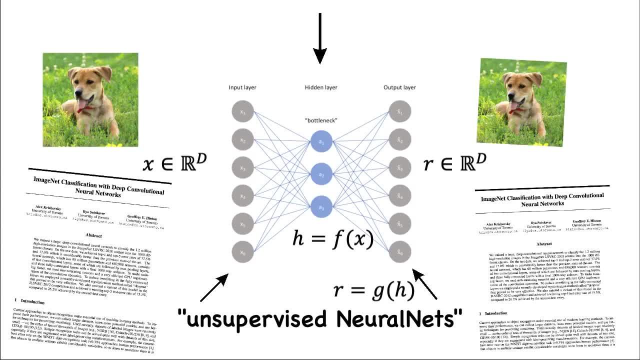 The output represents the reconstructed input, Hence it has the same dimensions. The objective is to learn a representation that will minimize the reconstruction loss. Learning these weights can be done with techniques like recirculation or backpropagation. However, there is a problem. A trivial solution would be a zero loss if we just copy the images. 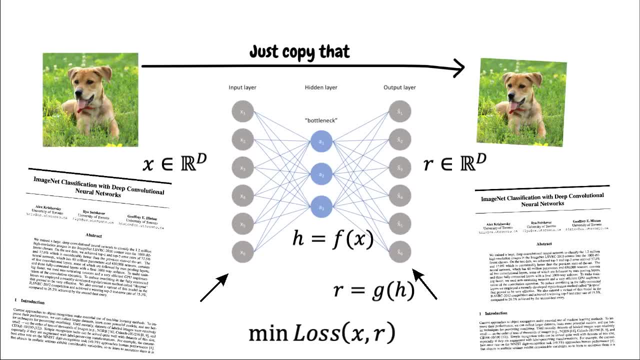 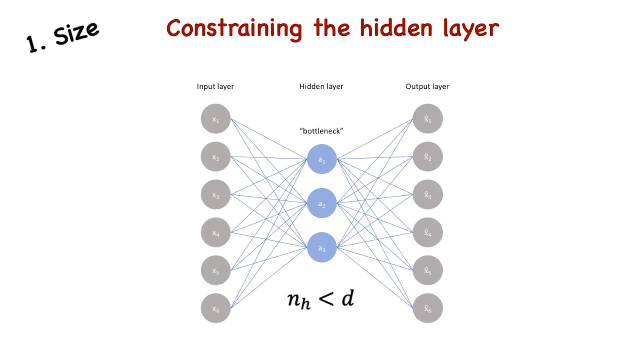 But this would mean that the latent layer doesn't really learn anything, which is useless. One way to work around this is to constrain the properties of this hidden layer, These properties being the size and activation. Consider size If the number of neurons in H is less than that of the input layer. 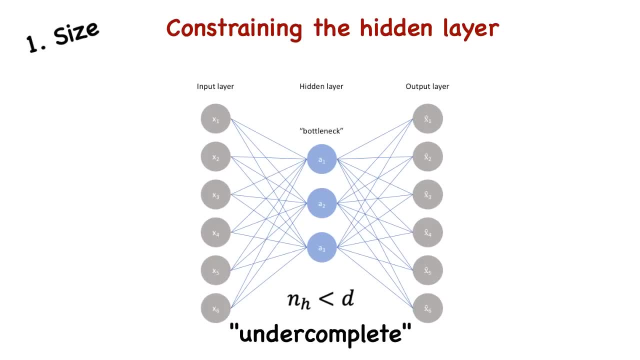 the autoencoder is set to be undercomplete. This is useful, as the network needs to learn latent representations within only a small set of neurons, so we're sure it's going to learn something. The second property is activation. If we don't use an activation function for the decoder phase, 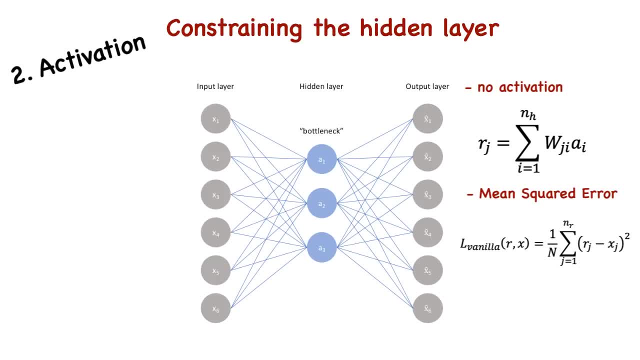 and the loss function is the mean squared error, then the results are similar to PCA principal component analysis, And so the latent representation of k neurons will represent the top k principal components. Adding a nonlinear activation in the encoder and decoder parts allow us to perform a nonlinear 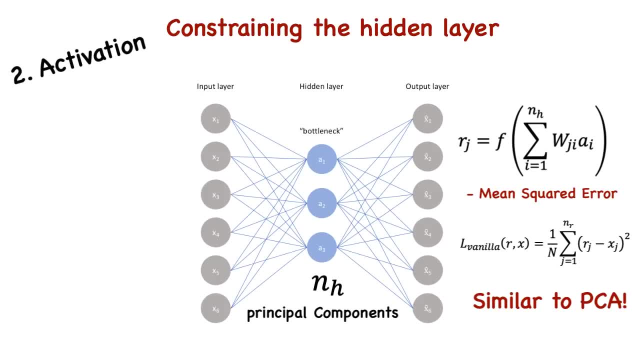 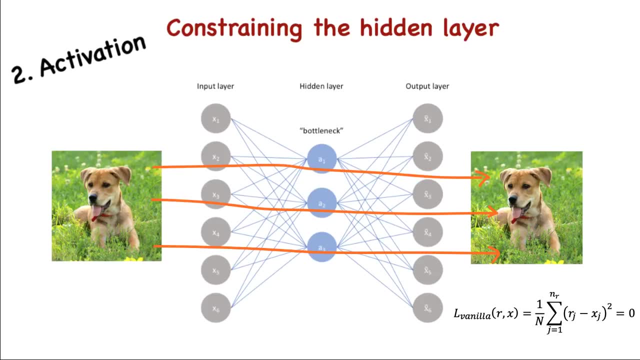 version of PCA. But then we come back to the same problem. If H is unconstrained, it will simply copy the input to the output, as that leads to a zero loss. We need to make sure that H is restrained to an extent for learning. 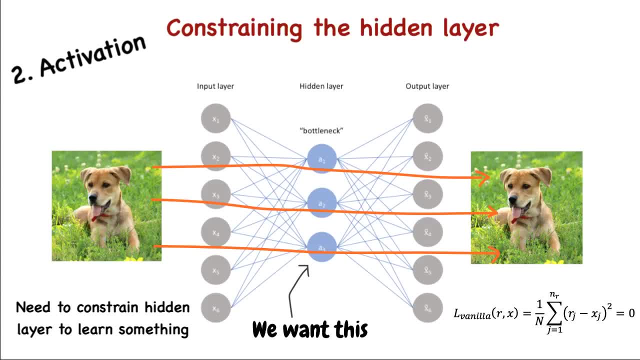 It is important to remember that we aren't too concerned about the output of the decoder, but more of the latent representation that the autoencoder learns Already. we can see a problem with this vanilla autoencoder. We need the latent feature vector space to be small and the encoder and decoder parts. 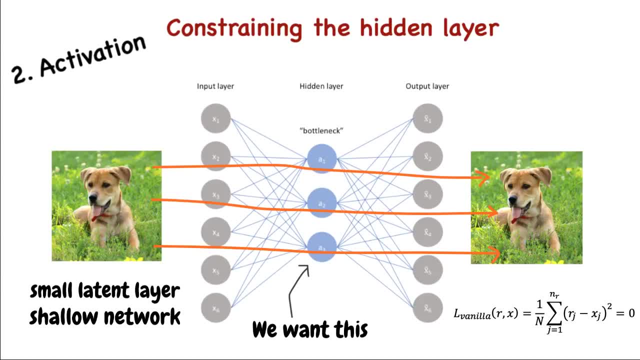 should be shallow. If not, the resulting latent representation becomes useless, as it simply copies the image. This means more complex data cannot be modeled accurately and we may end up with underfitted models. Ideally, we should be able to have a latent representation that is at least the size of 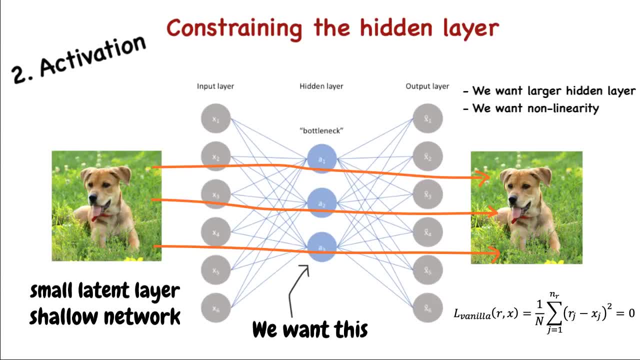 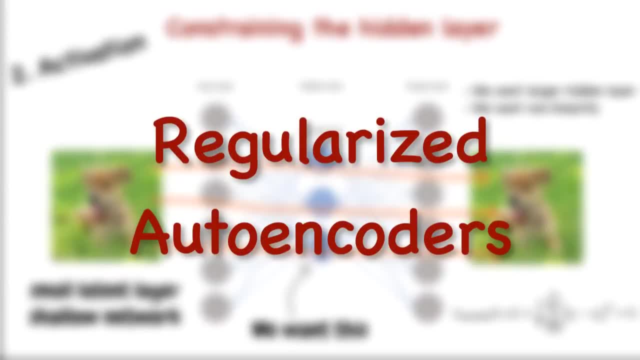 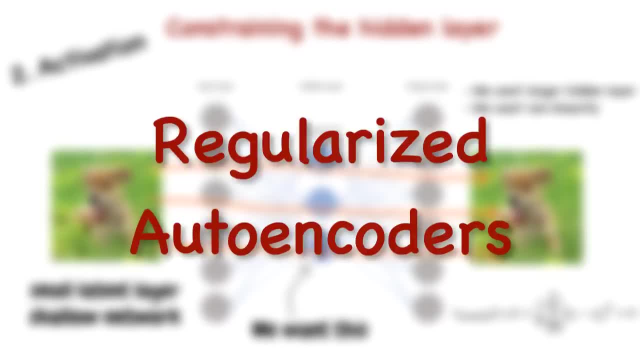 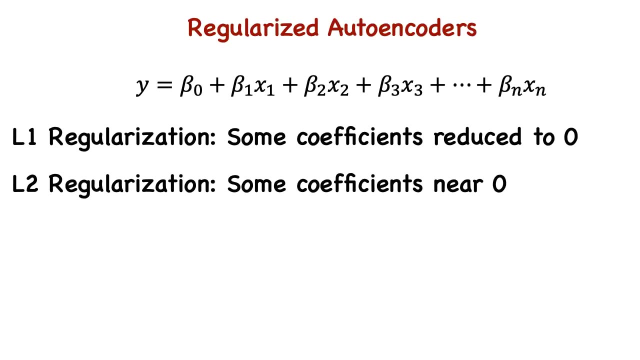 autoencoders but have a modified loss function. When you hear regularization, you're probably thinking of L1 and L2 regularization, where the coefficients are penalized to mitigate overfitting. We have a similar intuition here for sparse autoencoders. 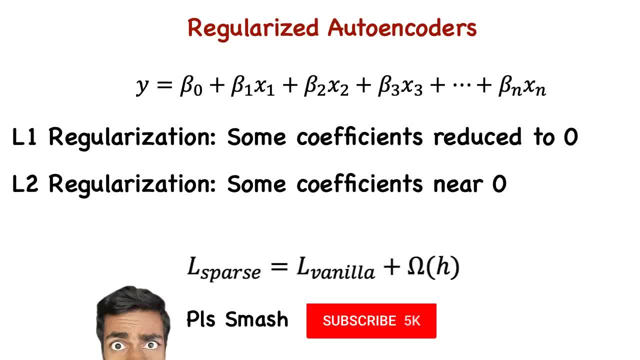 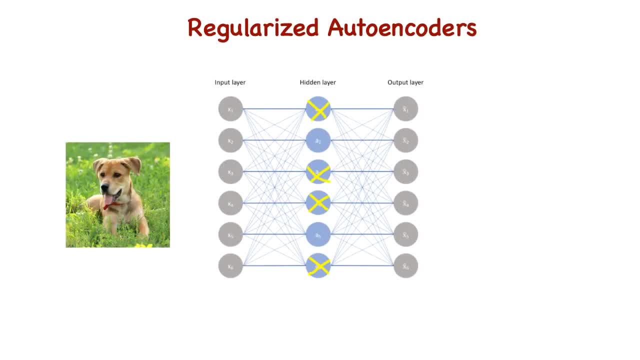 The overall loss contains an additional sparse penalty term on the code layer H. While thinking of sparsity, think most neurons are turned off. You can relate this to the concept of dropout in neural networks, where neurons are randomly turned off. This forces the network to learn. 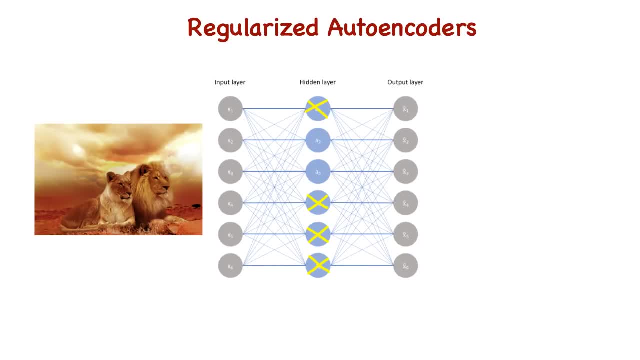 more accurate representations that better generalize training data. Let's say the hidden layer has a sigmoid activation. This means that the output values will range from 0 to 1.. We say a neuron is off if it is close to 0, and on if it is close to 1.. 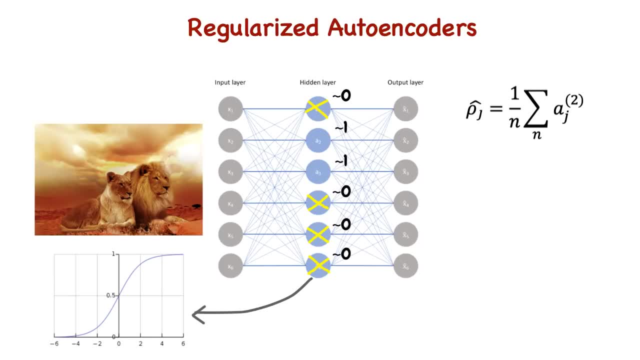 We impose a sparse loss function on the code layer H. We impose a sparsity constraint by making the average activation output of each hidden neuron some very low value, say rho j for the jth neuron. This rho j hat is the sparsity parameter. 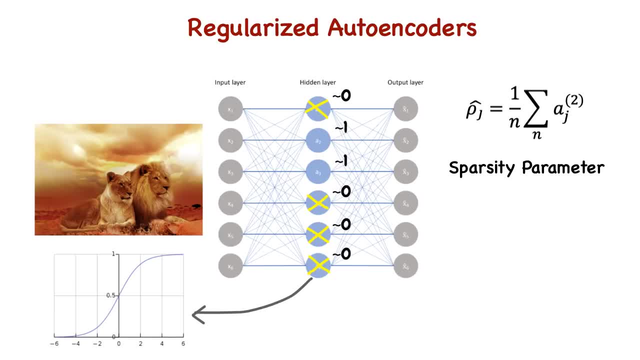 Now this notation may look a bit confusing. Basically, if we have n samples, each neuron in the hidden layer is activated to some extent. We want the average to be some low value. rho j I'll make the activation function a function of training examples as well. 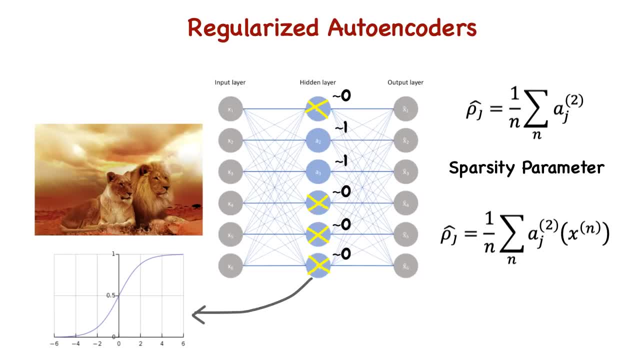 It's a fun compromise. if you want to say that as a merit of cheating- uh, you unter the function iserman. Well, here's the result. Using population, we're now able to estimate the activation of세요 above f to show that the activation of the jth neuron aj depends on the sample Xn. Note: it's just a function, not a multiplication with the input vector. We want it to be a very low value, like 0.05.. But we cannot just set it to 0.05.. It's an aggregate, after all, not a simple value. So we set rho j to 0.05, and penalize all neurons with a rho j hat that deviates from 0.05.. 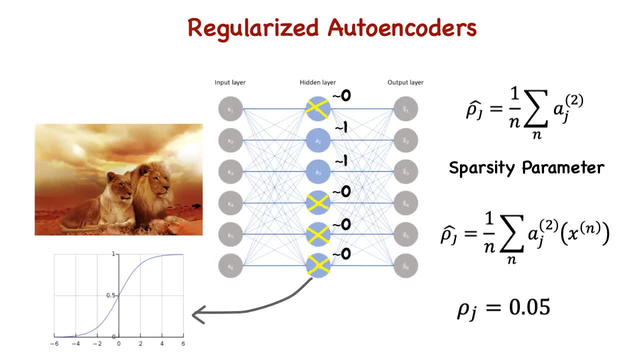 It's a simple benefit. so we beforehand choose the value of 0.05.. Not a right expression, Because we don't ог10 be calculated last time or deny the end of the way we get all neurons in the input with a rho j hat that deviates from this value. We can model two distributions, p and q, with the. 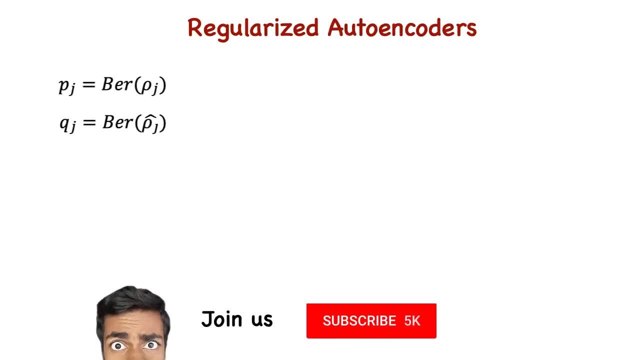 probability of success being rho j and rho j hat respectively. The idea is to ensure the predicted distribution is as close to the actual one, and we can model this with the KL divergence. Now, this is just one loss function that could work. just remember we are considering a sigmoid. 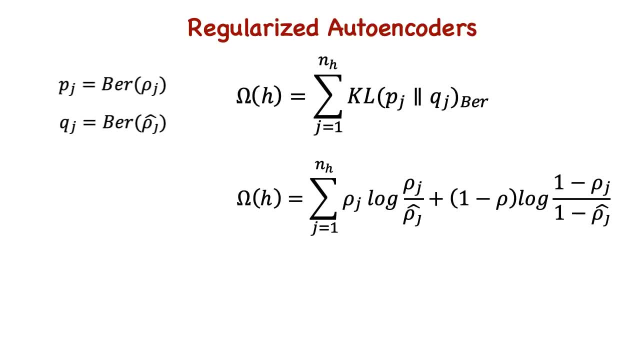 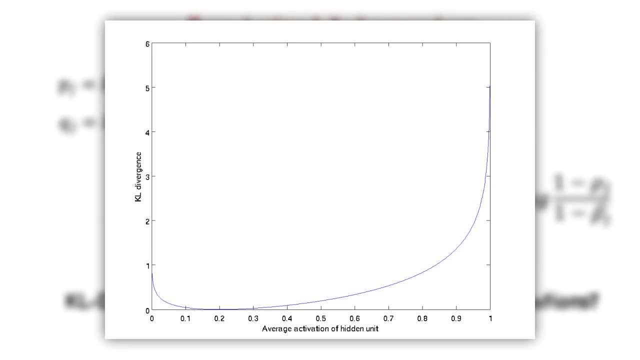 activation. This is equivalent to the KL divergence between two Bernoulli distributions, with the probability of success being rho j and rho j hat. By the way, KL divergence is a measure of difference between two distributions. ideally, we want to minimize it. This graph shows the KL. 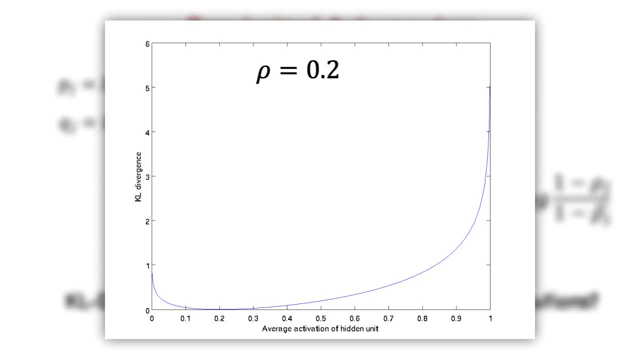 divergence. when rho is equal to 2 for a sigmoid activation, Clearly it's minimum. when rho is equal to rho j hat, We write the overall cost function as the sum of cost and current value of the loss function and we can see that the loss function is equal to rho j hat. 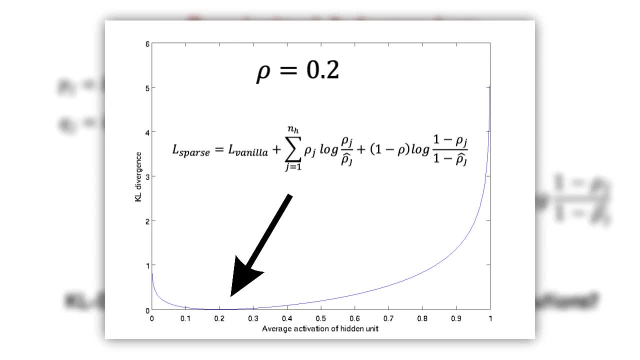 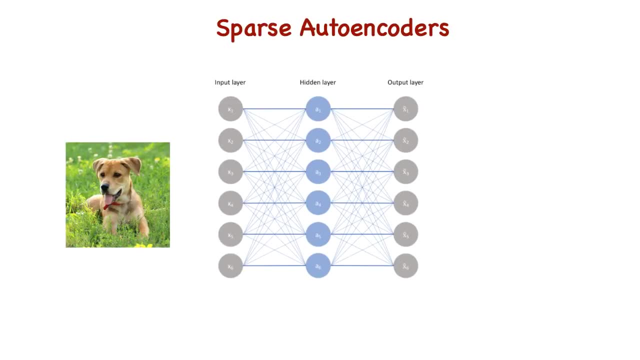 So how exactly does sparsity help? We can take a look at the network that learns visually. Say we have an autoencoder whose input is a set of 10x10 images- so that's a 100-dimensional input- and say that we use a hidden network of size 100 as well. After training, we want to visualize the 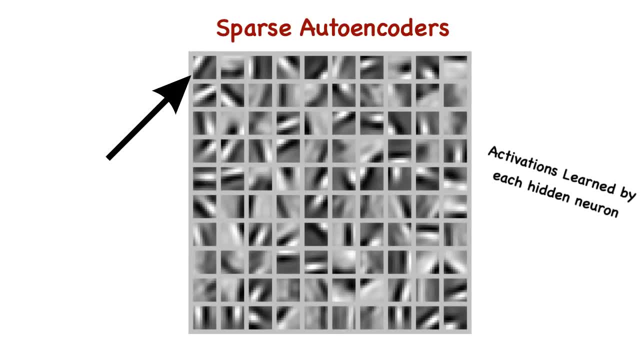 components as shown here. Consider the top left corner, which was learned by the first neuron. This neuron learned to detect diagonal edges. All neurons like so learn to detect edges of different orientation, so together they learned a very effective representation. Another type of regularized encoder are denoising autoencoders. 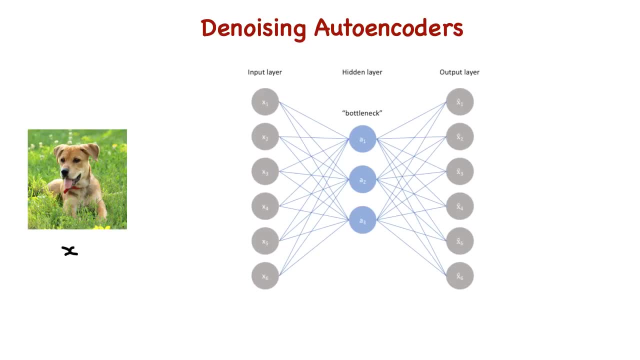 Autoencoders learn a latent representation from the input text in an unsupervised way. Denoising autoencoders can be used to detect diagonal edges, and they can detect diagonal edges of different layers. Autoencoders learn such a representation from a corrupt input. This allows for a better 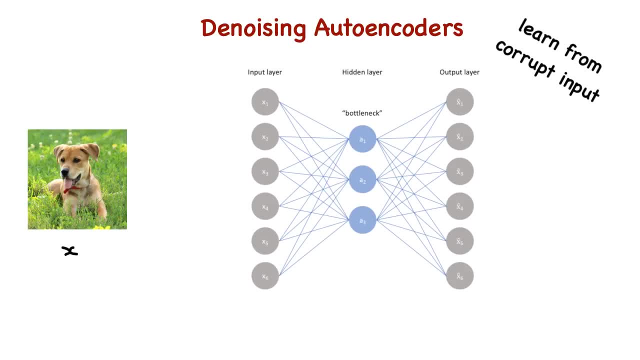 generalization So you can take the input x and add some noise to it. The resulting corrupted input is x dash or x prime. The hidden layer can no longer simply copy the input to the output. hence it is forced to learn some latent representation For the most part until now. 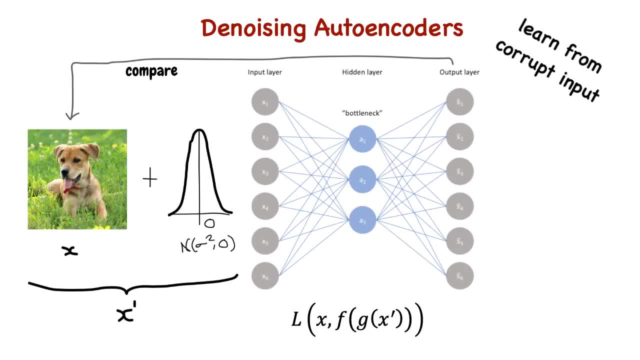 we've only been talking about autoencoders with a single hidden layer for the code layer, The single input layer for the encoder and a single output layer for the decoder. Such a shallow network can actually be quite useful. You can attribute this to the universal approximation theorem. 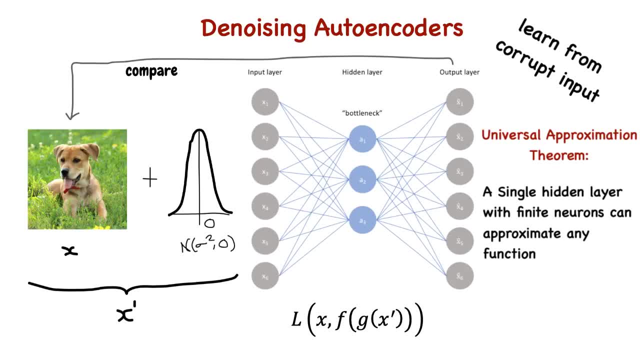 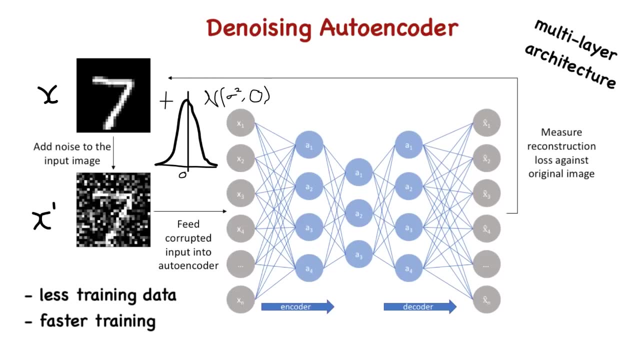 In neural net theory. a neural network with a single hidden layer and a finite number of neurons can approximate any function with assumptions of its activation. However, there is nothing stopping it from creating deeper architectures. This allows faster training times, as we don't need as much training data for 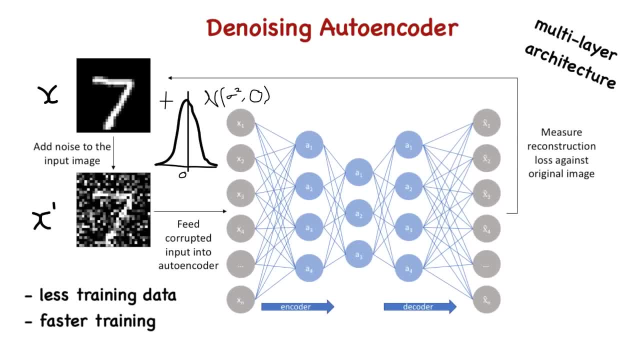 a good generalization. Hope you can now see how autoencoders can be used in data transfers across a network- The example application that we talked about in the beginning of the video. They can also be used in instance segmentation, Swapping out fully connected layers with. 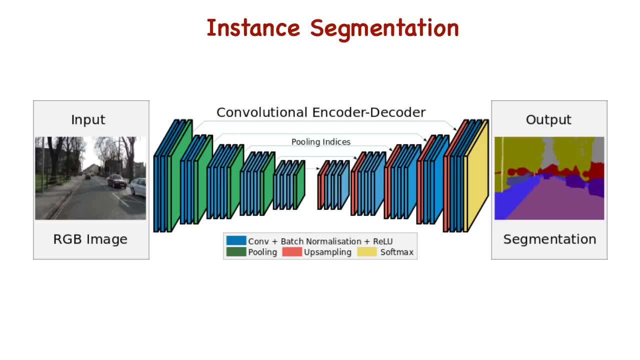 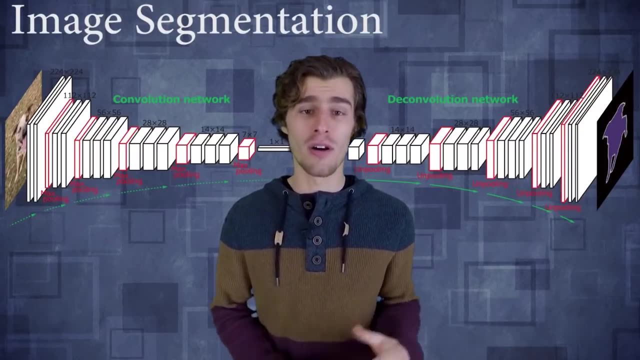 convolution layers. the autoencoders can take image inputs, preserving spatial representation, But instead of the original image, we aim to output a semantic, segmented counterpart outlining the contours of interest. For example, this tech can be used in self-driving cars to segment different objects of interest. 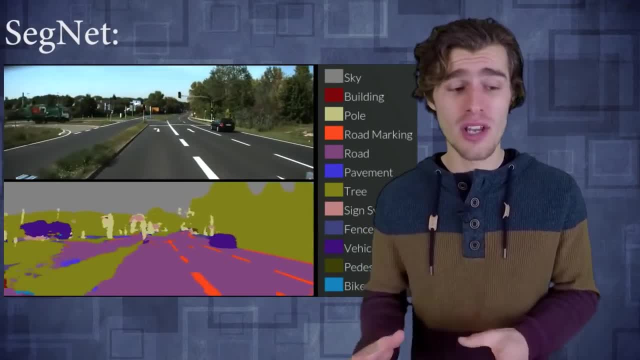 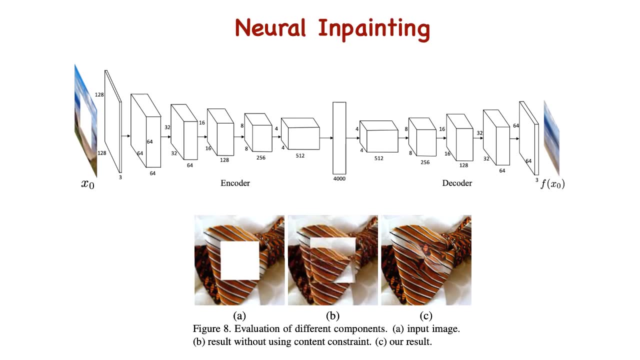 Xander on Archive Insights does a pretty good job of explaining this on his variational autoencoder video, so check that out. Another application is neural inpainting. Instead of adding noise to autoencoders, you can remove rectangular sections from an image and try to reconstruct the original.